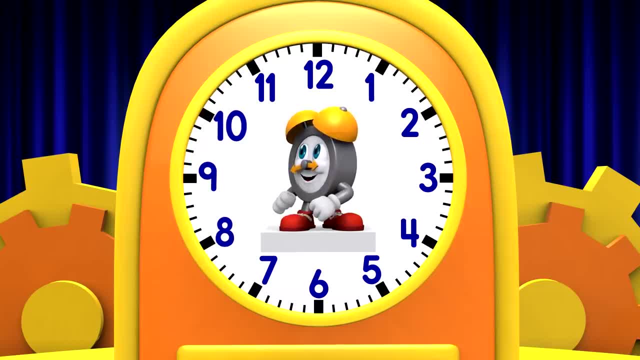 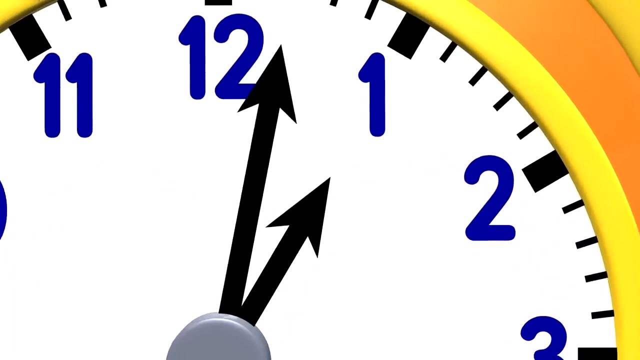 Seven, Eight, Nine, Ten, eleven, twelve. One, two, three, Four, five, six, Seven, eight, nine, Ten, eleven, twelve. Running round the face are at least two hands. The short one moves most slowly as the hour demands. 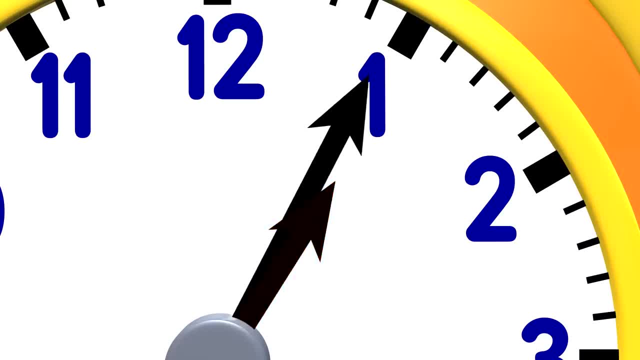 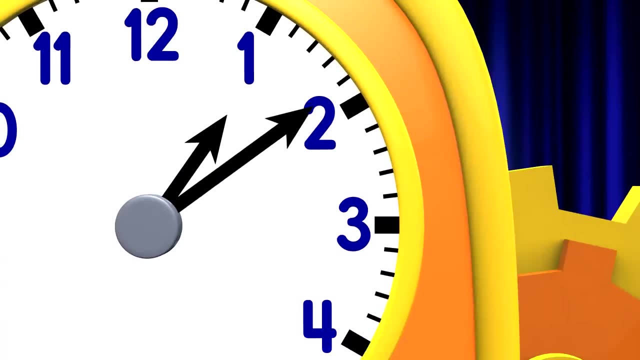 Because the short's hands are the slowest. First hand is the hour hand. He's so slow I could slumber. He takes a whole hour just to reach each number. The long hand is the minute hand. She moves a little faster. 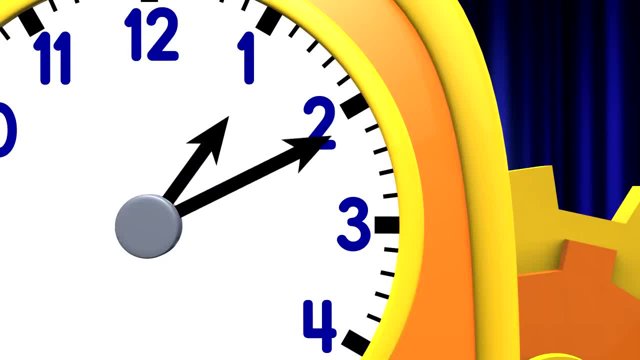 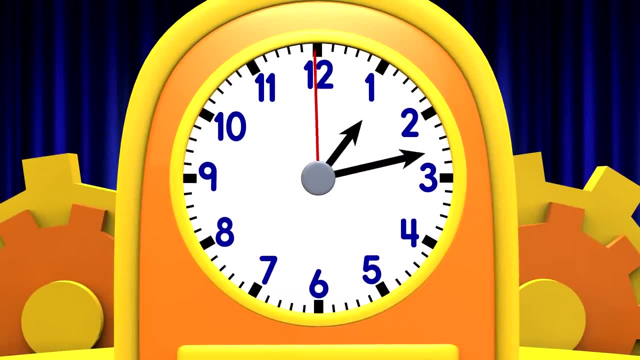 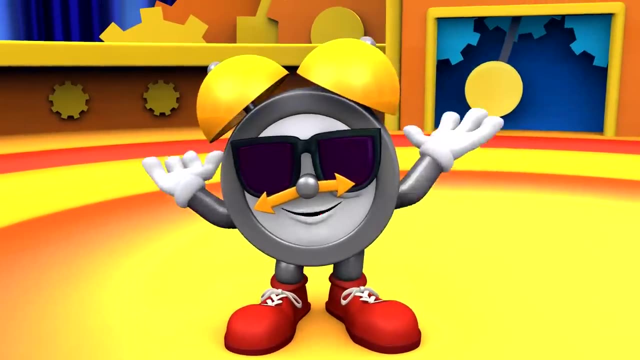 Every five minutes she gets a number past her. Some clocks have another hand that speeds around the face. This thin one is the second hand. Now pump up the bass. Yeah, Pump up the bass. Pump it up now, Ooh, Ooh. 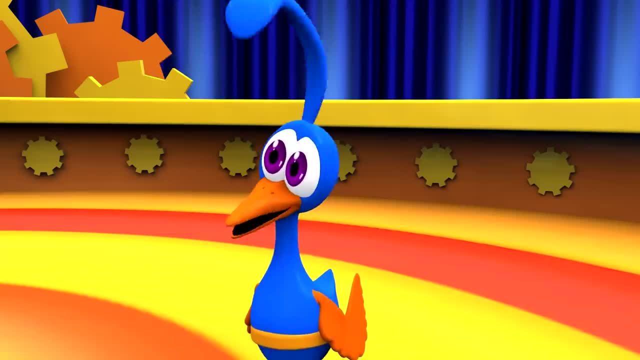 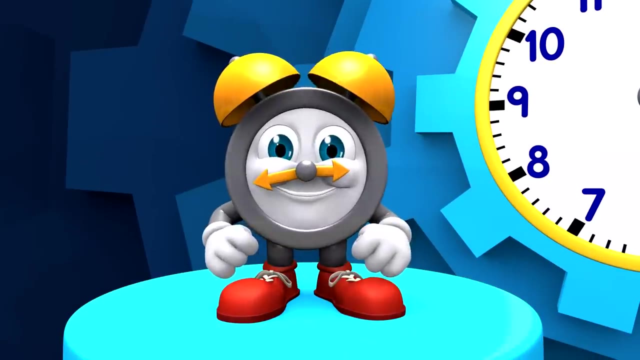 Come on, Cuckoo. Okay, okay, calm down. Oh sorry, Cuckoo, I guess I lost track of time, Ha ha. Oh, brother, Speaking of time, Now you know the parts Of the clock that you read. 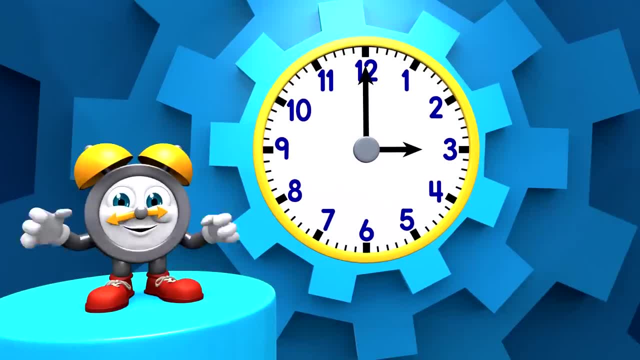 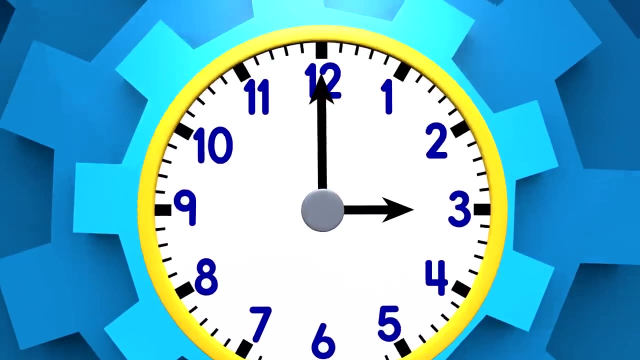 In order to tell time, A clock is what you need. Let's start out easy Telling time to the hour. I'll teach you a cool trick that will give you the power When you see the minute hand pointed straight at the top. 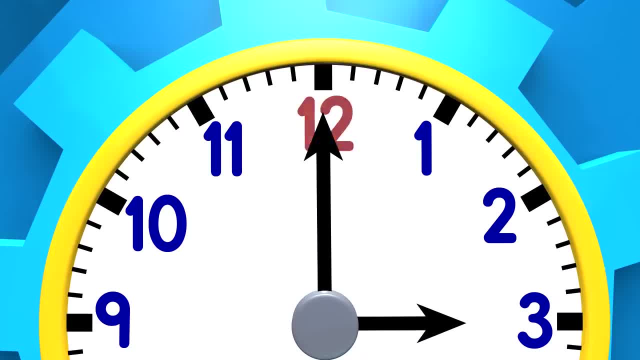 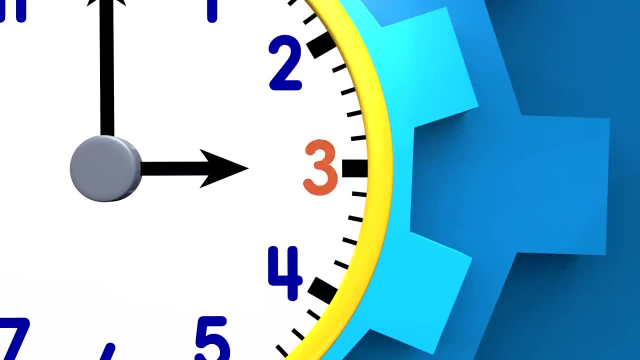 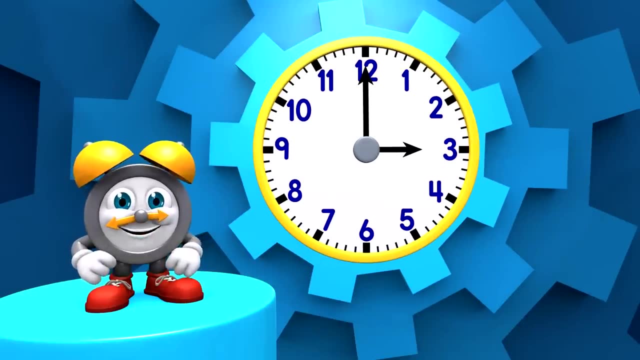 It's on the number twelve. So say the word o'clock, Next check out the number, The hour hand points to Then put that number with o'clock. That's all you have to do. Let's try a few examples. Just take a look at these. 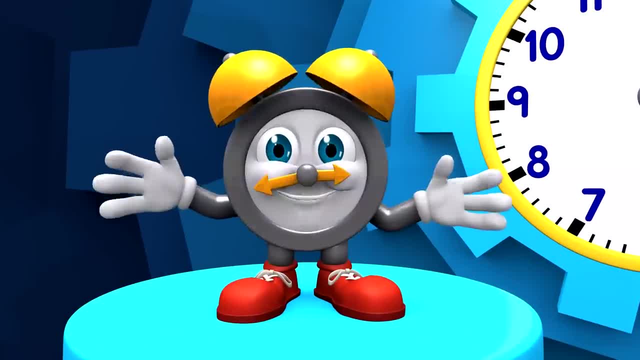 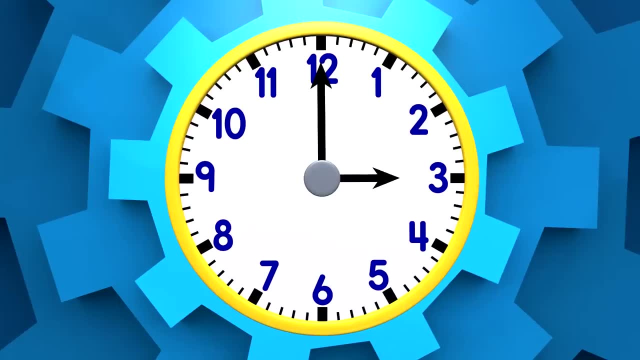 And say them out loud As quickly as you please: One o'clock, Two o'clock, Three o'clock, Four o'clock, Five o'clock, Six o'clock, Seven o'clock, Eight o'clock, Nine o'clock, Ten o'clock, 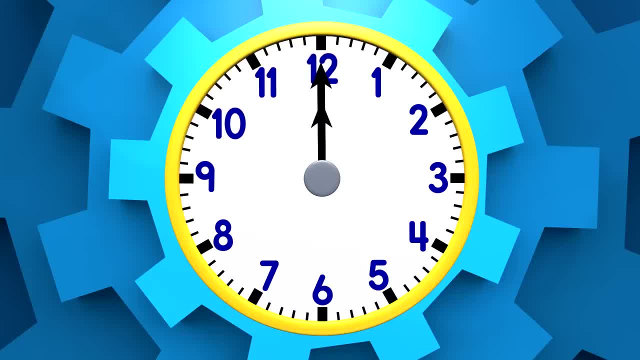 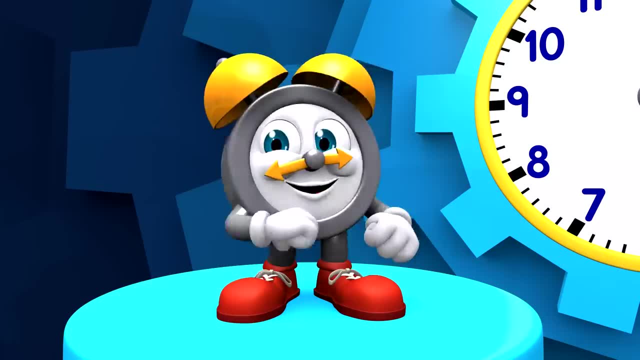 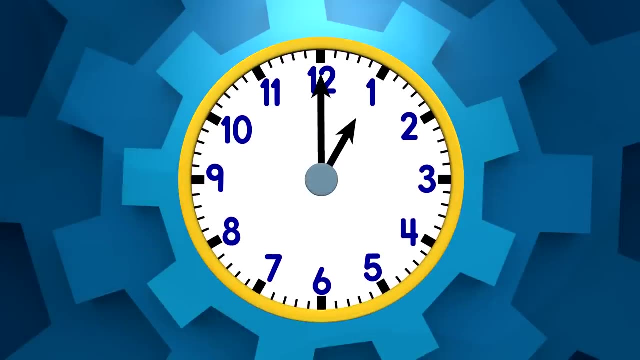 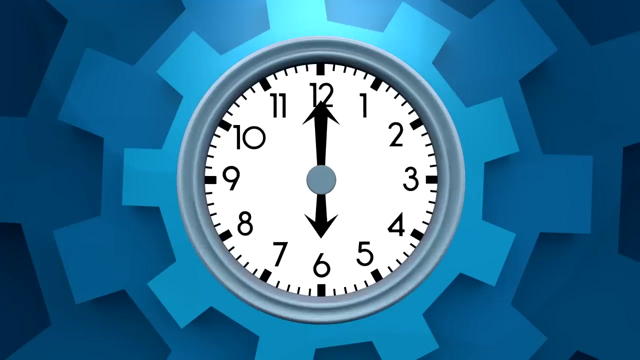 Eleven o'clock, Twelve o'clock. Now let's try some other clocks, Like ones that you might see, So you get some more practice. Say these times with me: One o'clock, One o'clock, Three o'clock, Six o'clock. 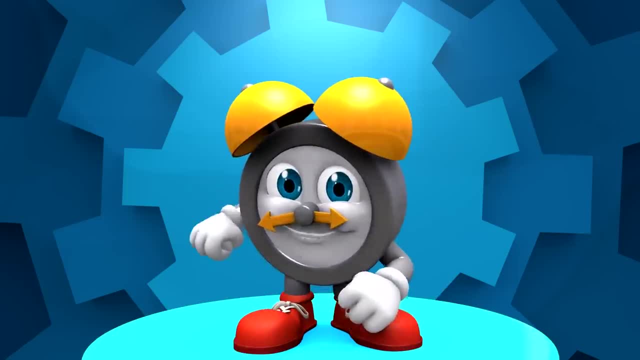 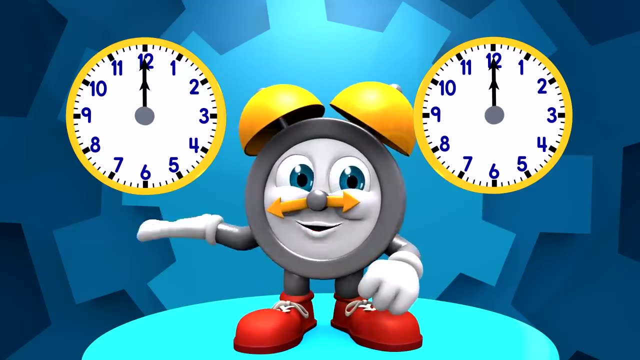 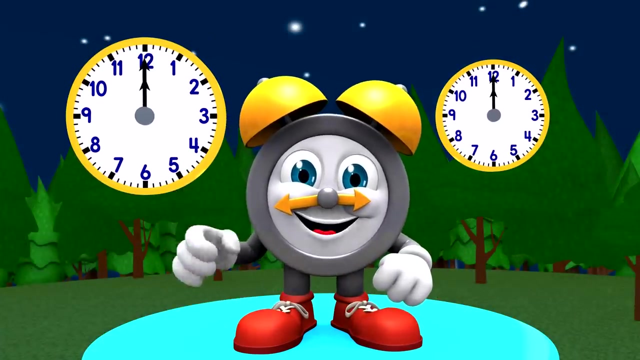 Eleven o'clock. Some of you have noticed something a little strange. It seems we have two of each hour in each day. The first twelve o'clock Comes when it is night. This is twelve am And also twelve midnight, Twelve hours later. 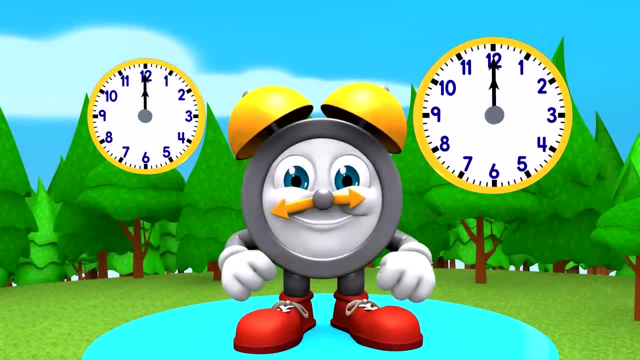 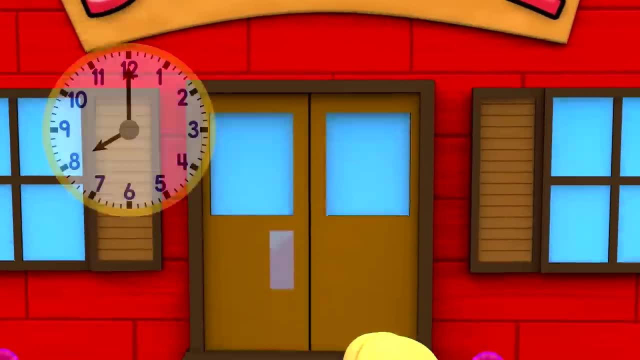 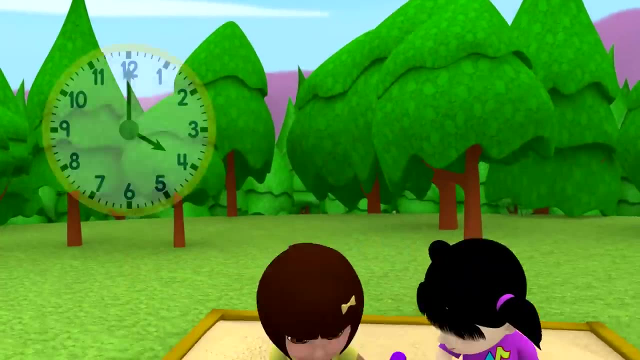 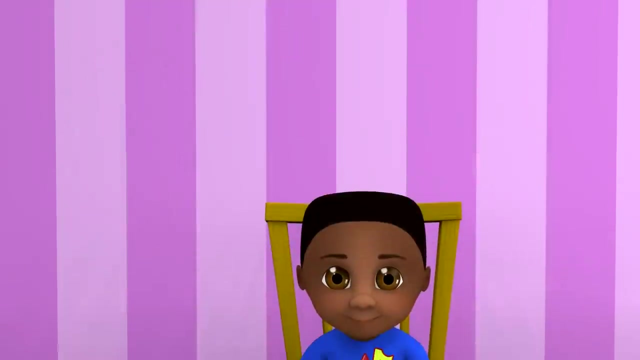 It is noon Or twelve pm. Let's look at some examples now And join along with them. Eight o'clock am Is the start of my school day. Four o'clock pm Is the time for friends to play. 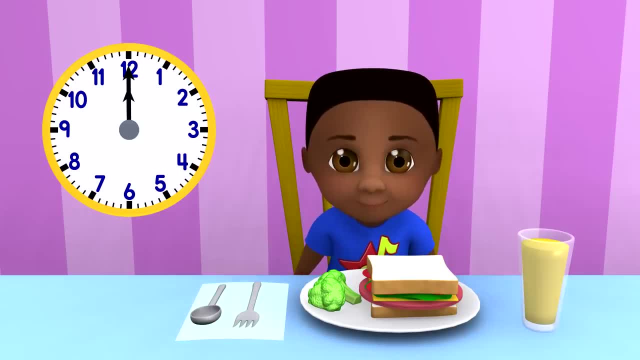 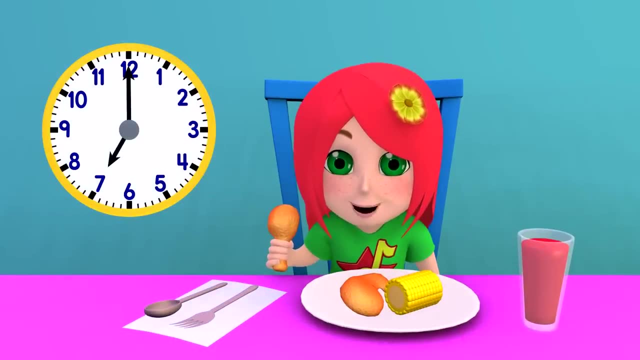 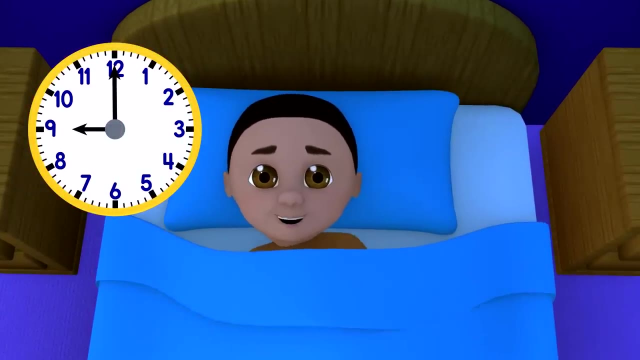 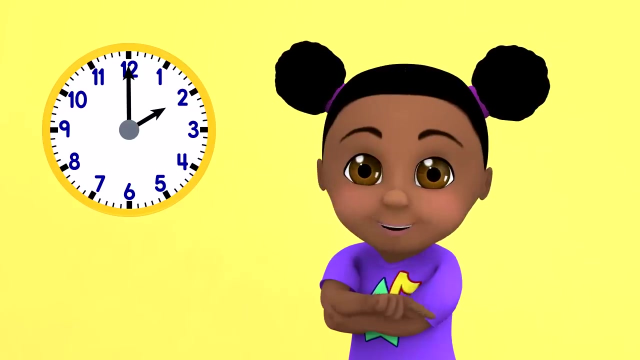 Twelve o'clock pm Is the time to eat some lunch. Seven o'clock pm Is when my dinner gets munched. Nine o'clock pm Is when I need to be in bed. Two o'clock pm Is when I think of what my teacher said. 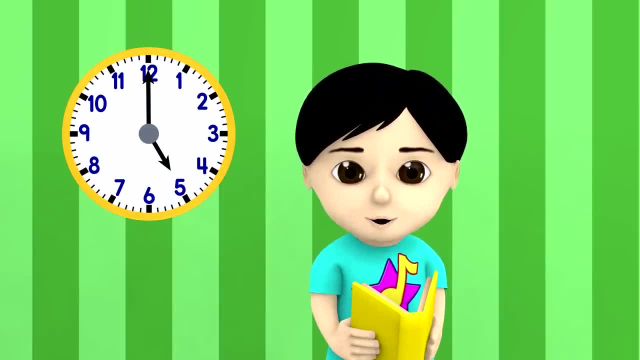 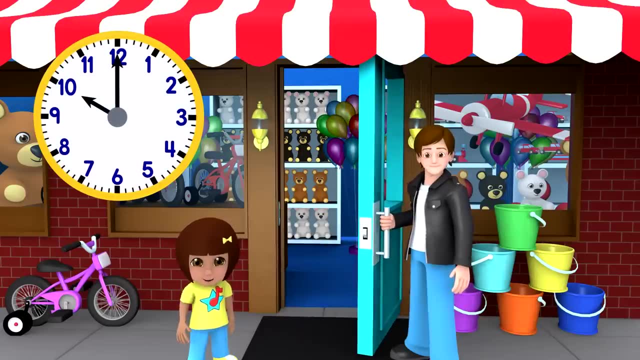 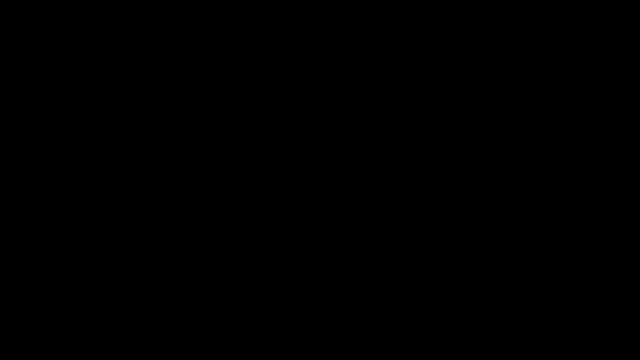 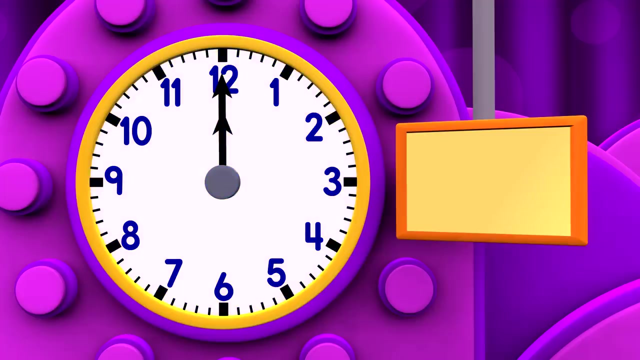 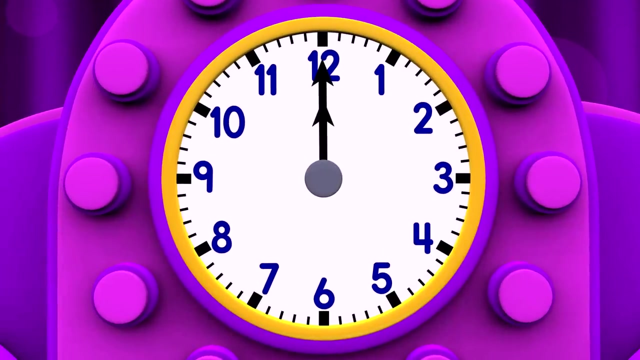 Five o'clock pm Is when I do homework and chores. Ten o'clock am Is when they open most stores. Since one whole hour has sixty minutes, Half an hour has only thirty minutes in it If you start on the hour. 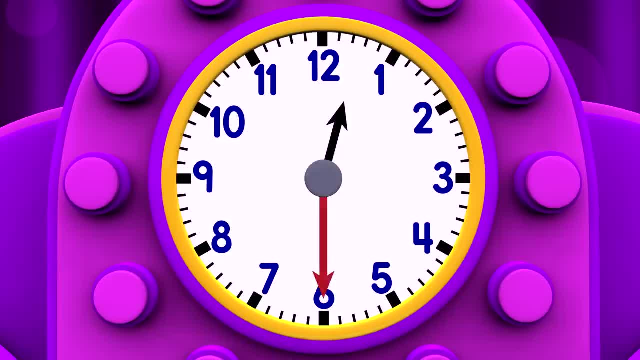 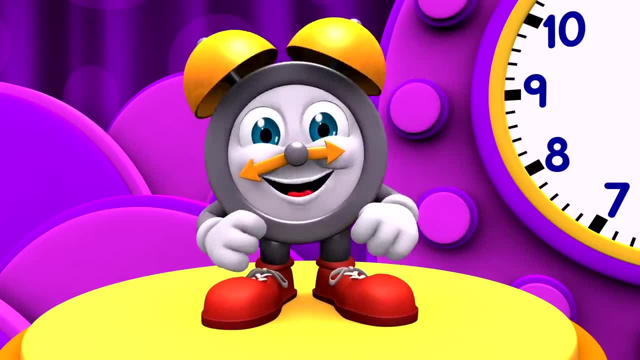 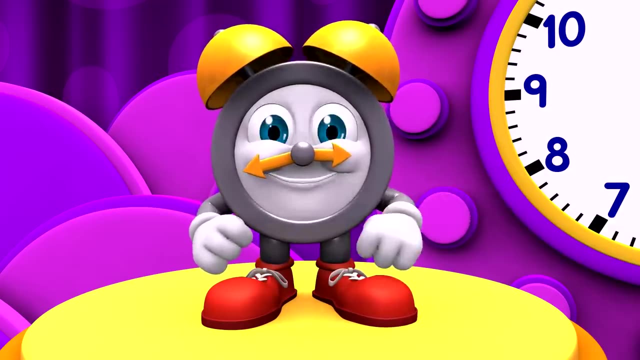 And go halfway around. The minute hand will be on the six Hanging upside down. Now you might ask Where will the short hand be. I can tell you now. It's quite easy. The hour hand will be Halfway in between. 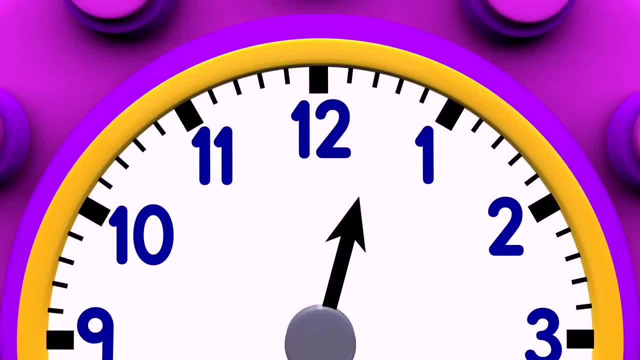 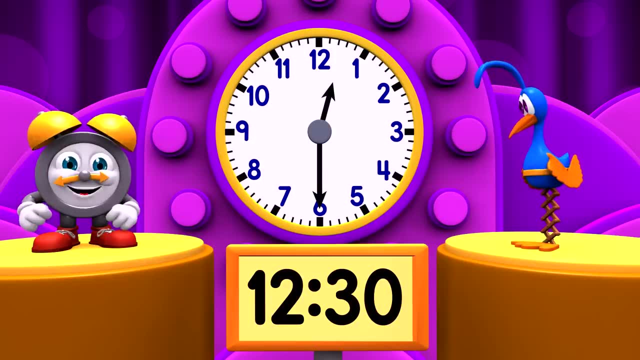 Two of the numbers Somewhere around the ring. Whichever of the numbers, The hour hand's just passed Is the one you say out loud, With thirty at the last. Well then, Show us how to do it. Okay, Don't get your feathers ruffled. 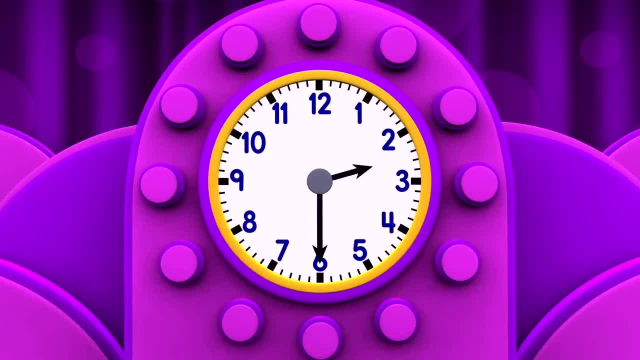 One, thirty Two, thirty Three, thirty Four, thirty Five, thirty Six, thirty Seven, thirty Eight, thirty Nine, thirty Ten, thirty Eleven, thirty Twelve, thirty. Okay, Timothy, So when I hear people say It's half past seven, 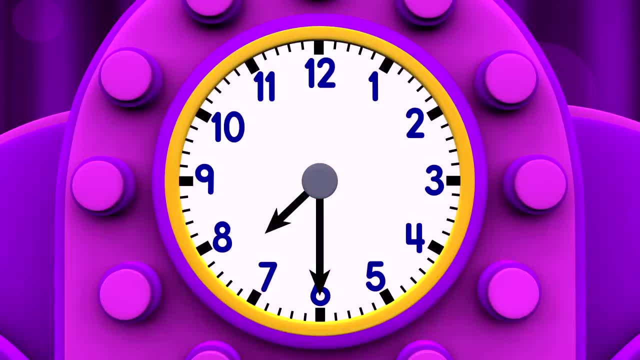 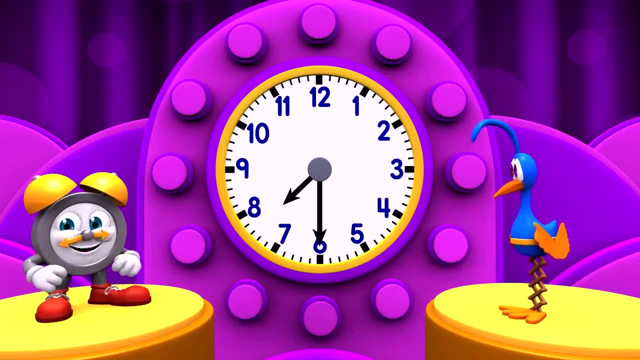 Does that mean That the minute hand is on the six And that it's seven thirty? Wow, Cuckoo, You catch on really fast. They say half past Because the hour hand has traveled Halfway past the number before it. 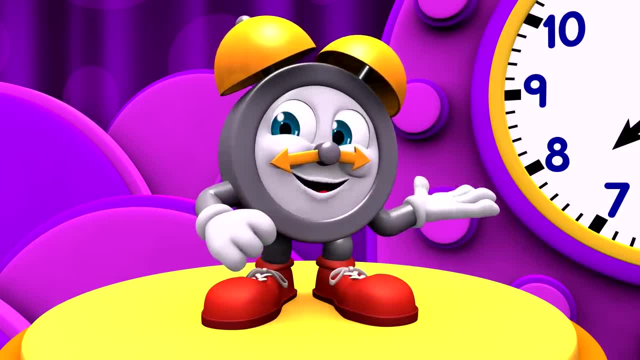 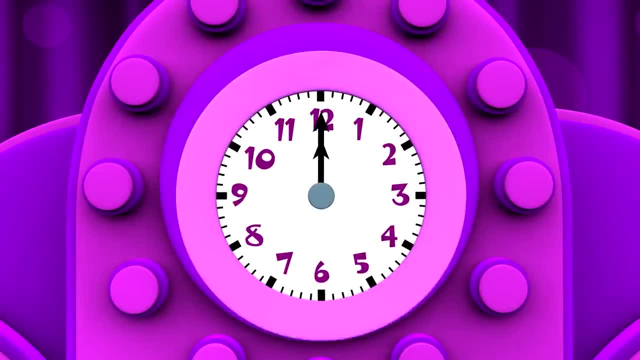 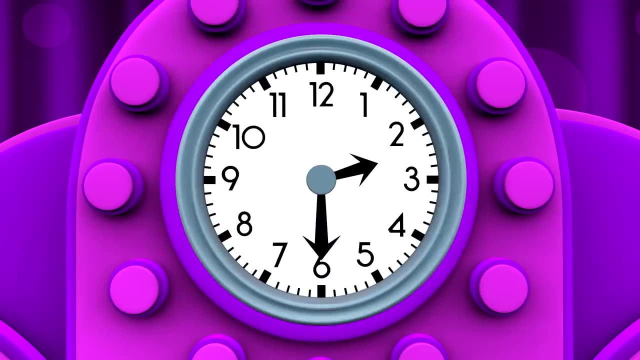 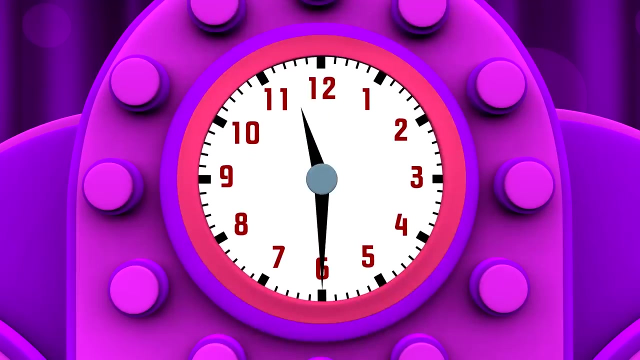 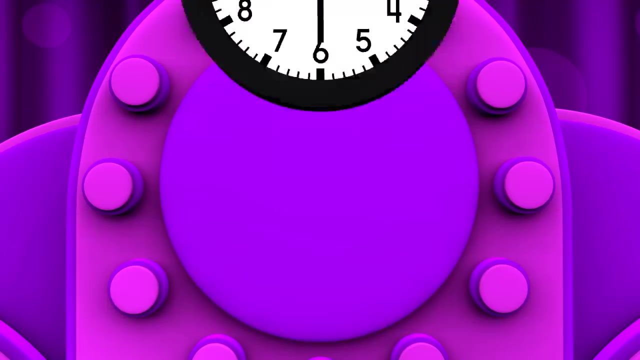 Let's look at some more clocks. Read the times on these clocks with me: Eight thirty Or half past eight. Twelve o'clock. Two thirty Or half past two. Eleven thirty Or half past eleven. Nine o'clock One thirty.